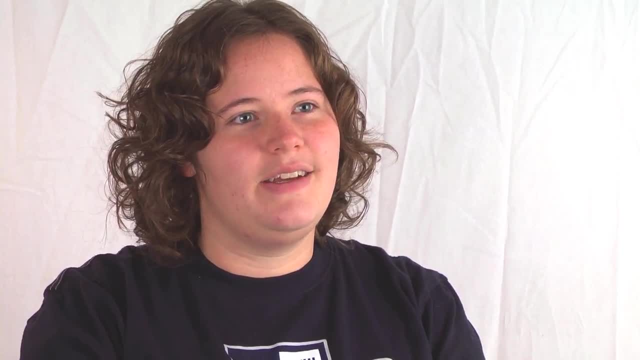 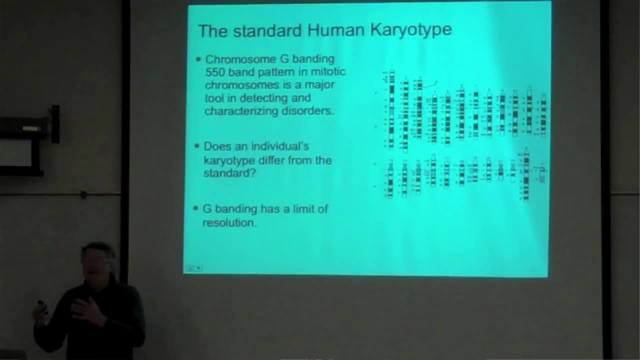 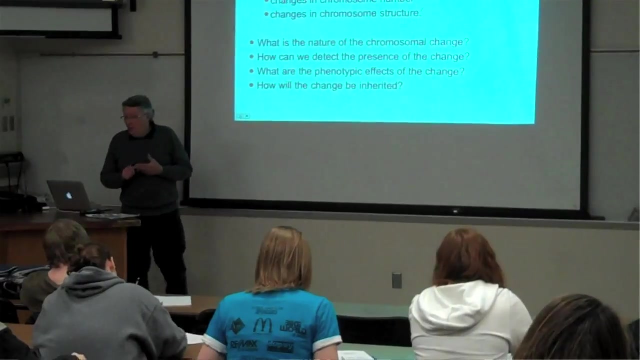 so it has more of a bioinformatics approach and different databases to search and how you would go about analyzing the genome Medical genetics. it's taught by Jack Gurtin and we've basically just been going over basic information regarding genetics and how it affects the genetic structure of the. 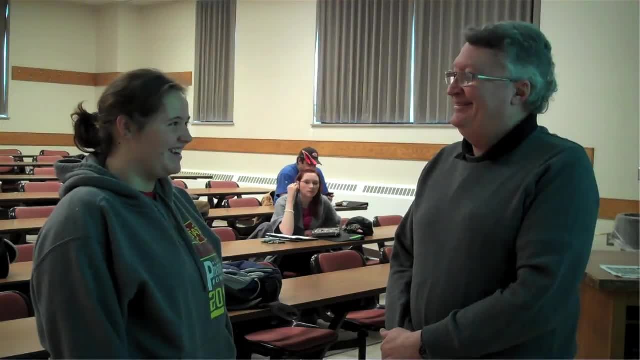 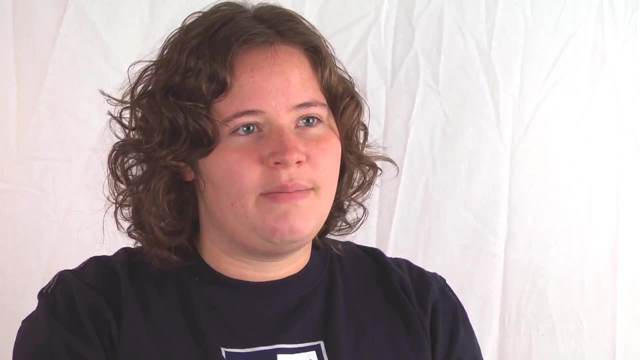 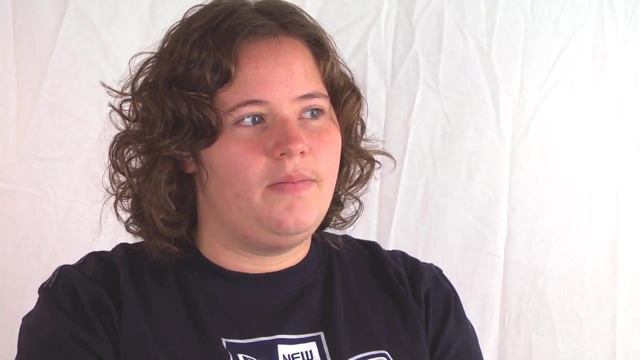 genome and the different diseases that are out there, and I was able to do a mentoring project in the spring semester and so I got to know the lab setting a little bit and sort of get my hands wet as far as lab experience goes. and then I am now actually employed at that same lab. I do things with cell culture. 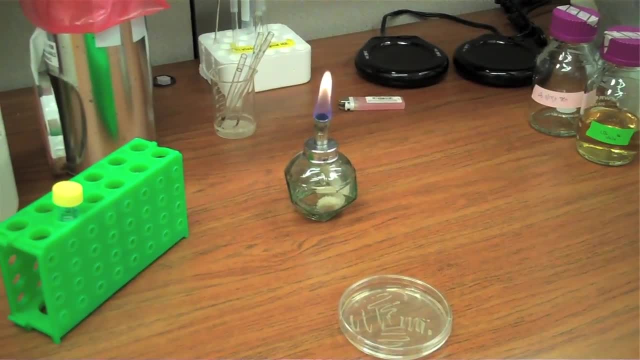 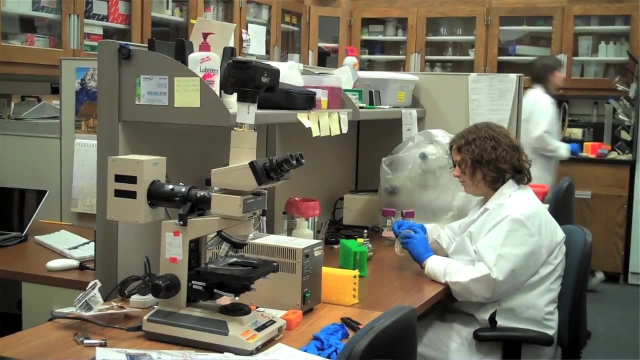 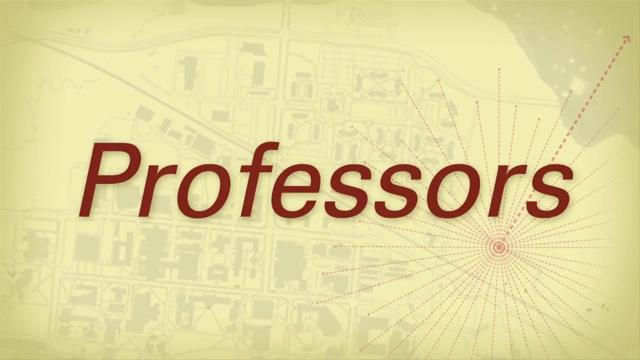 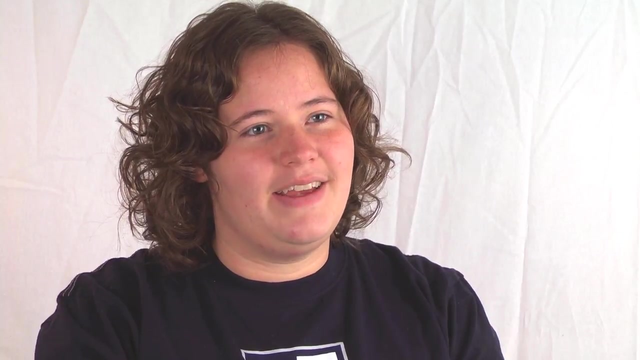 streaking plates, preparing media to put on the plates, feeding them, and just I help out with whatever procedures that they're doing for the day. Reverse transcriptase RNA purification gel extraction, Dr Cho, as I mentioned, I worked in his lab as a freshman, just as taking a. 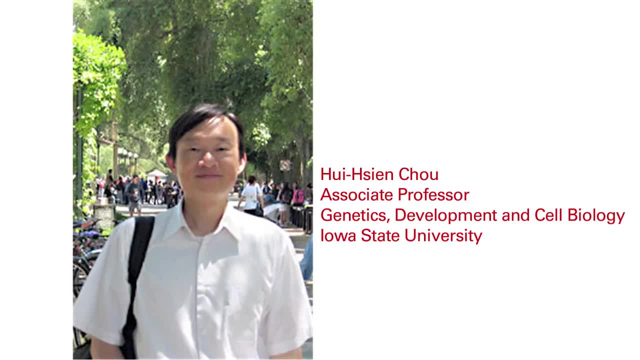 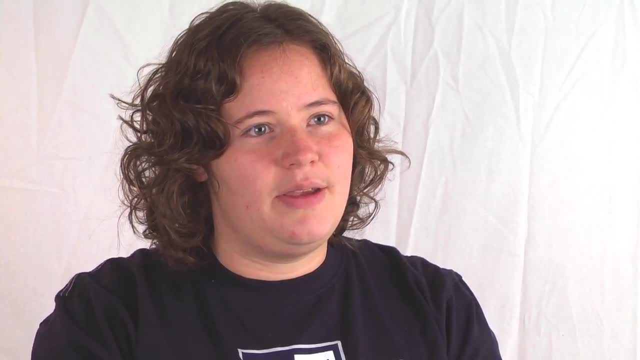 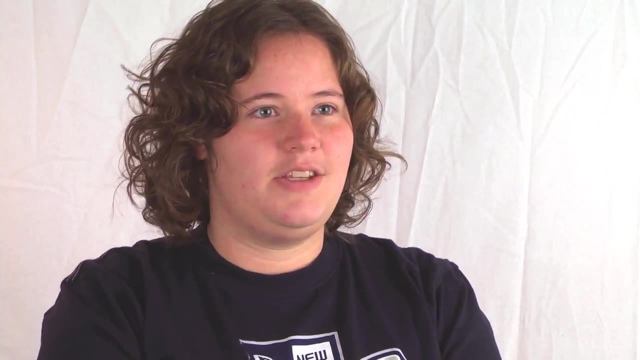 one-credit course and then that next year he co-taught one of my classes and after having had me in class and seeing me participate in his lab, he really he thought I was a really good candidate for a job there. so he gave me a job at the beginning of this year and I've 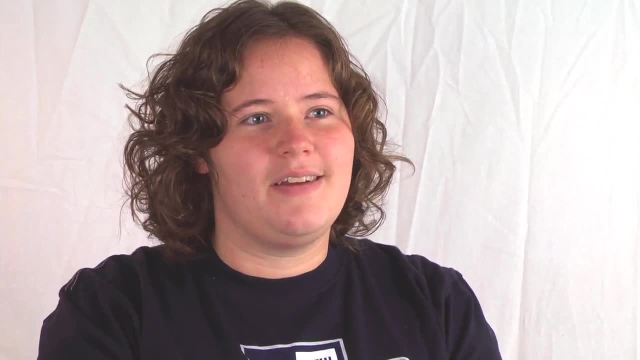 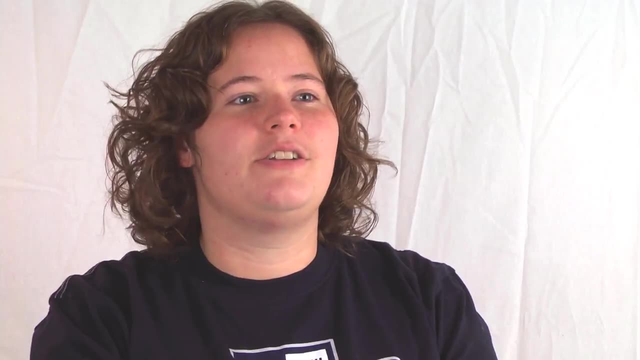 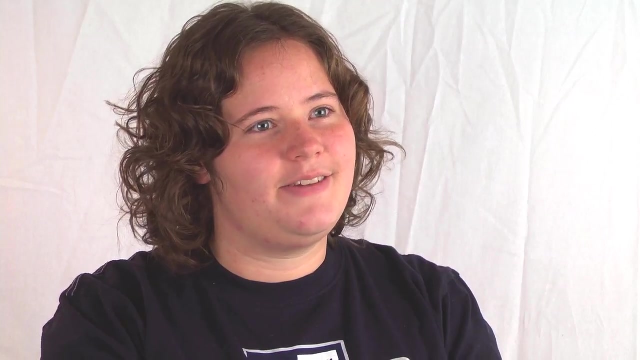 worked there since. So he sort of taught me new tools to use in the bioinformatics field and giving me advice on graduate schools and applying for internships, and he's been able to write letters of recommendation for me. Karen Dorman is her name and I go to her at least. 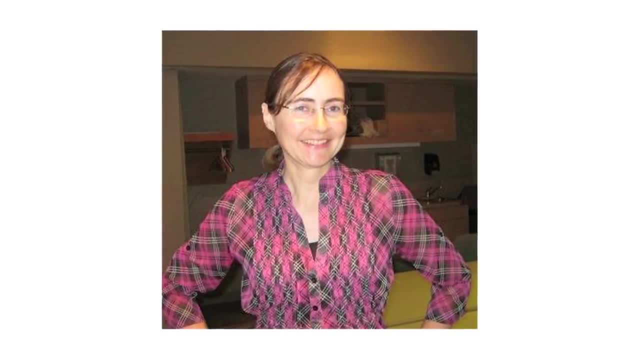 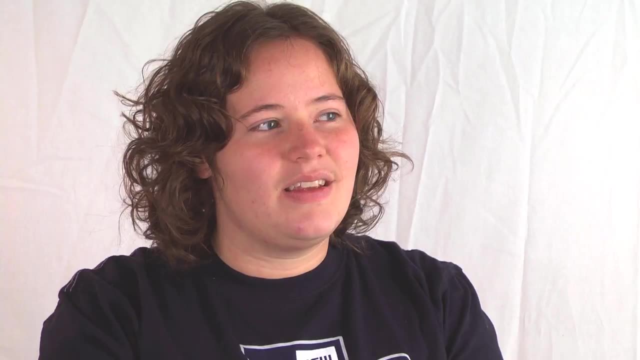 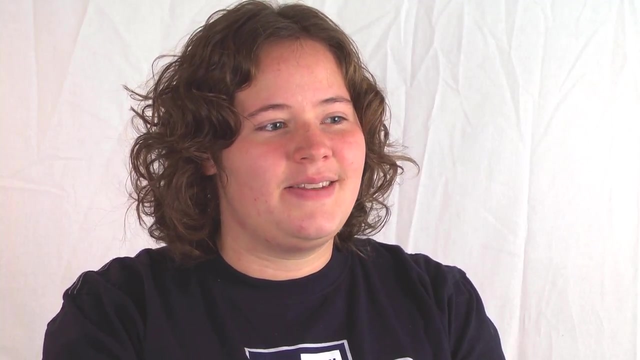 once a semester, sometimes more. She helps me make sure that I'm taking all the right classes that I need to take so I'll graduate on time, and she's usually pretty good about emailing me back and helping me with whatever else it is that I need- Studying abroad, information or applying to internships, graduate